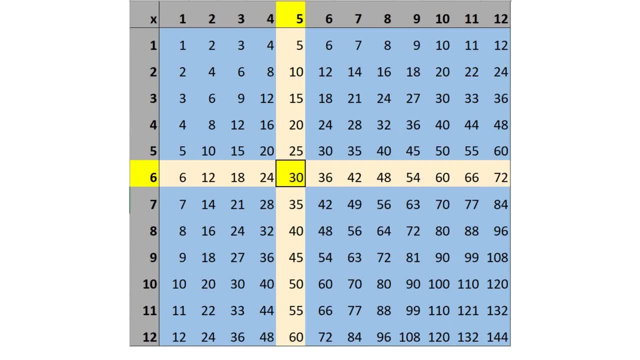 They're 30. The 5 comes down and the 6 goes across and we reach the answer 30. Yes, Good, And then let's just try it the other way around. If I went down the 6 column and along the 5 row where they intersect, I get to. 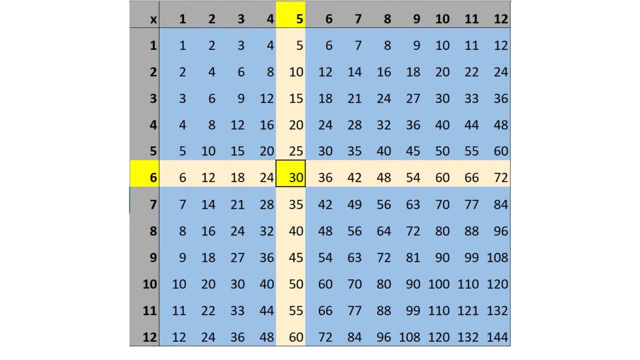 30.. 30 as well, So you can see 30 is in both of those places. Yes, And this multiplication table can be used for looking up answers to multiplication problems, in this case up to 12 times 12.. Yes, 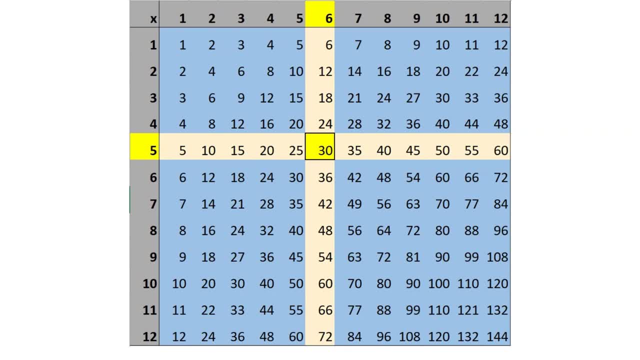 Now that's what people call the multiplication table, And it can go bigger than that. You don't have to stop at the number 12.. You could go on to the number 20 or the number 100 or even further, And the multiplication table would just keep getting bigger and bigger. 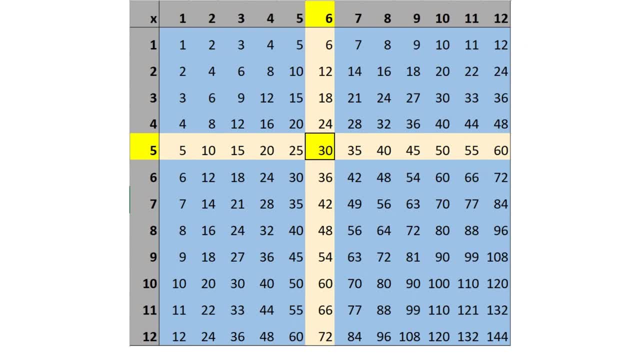 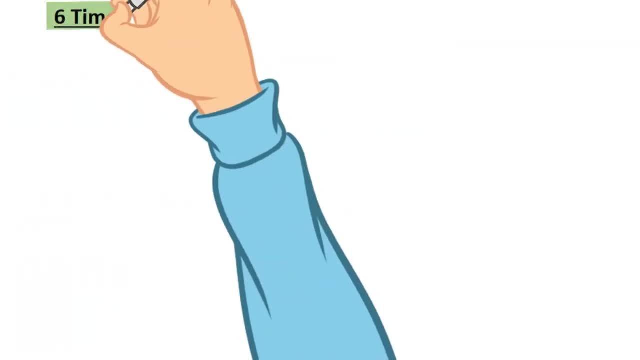 And when people refer to multiplication tables, what they mean then is stuff like this: Here's what we call the 6 times 12.. It's a table. So you've got 1 times 6 and the answer 1 times 6 is 6.. 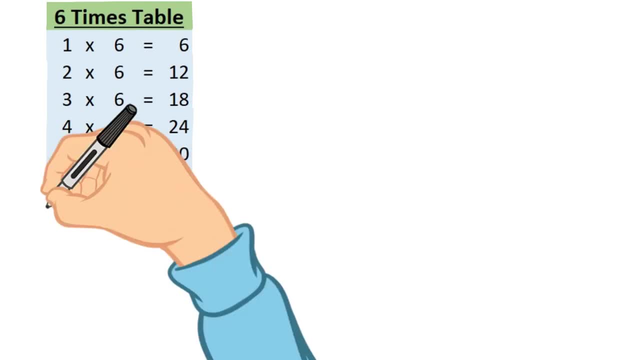 2 times 6 is 12.. 3 times 6 is 18.. 4 times 6 is 24.. So that's a times table that just works on problems that are something times 6.. And you'd have that alongside, for example, here the 7 times table. 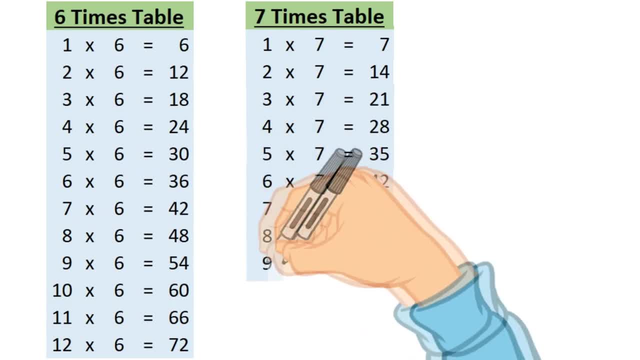 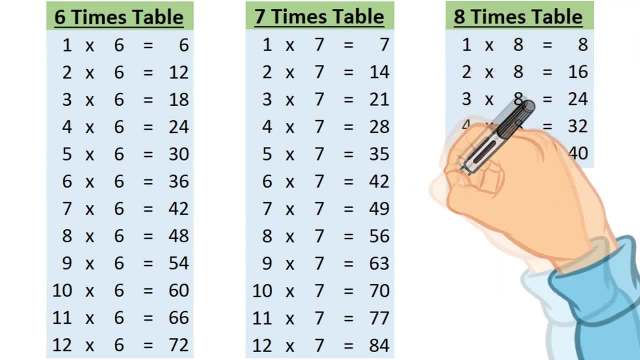 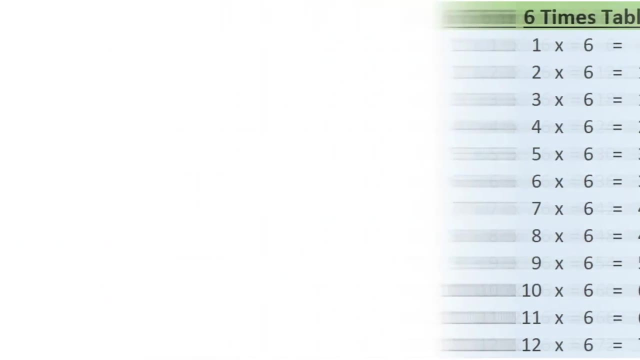 1 times 7 is 7.. 2 times 7 is 14.. And 8 times table: 1 times 8 is 8.. 2 times 8 is 16.. And so on, And these are the answers that you'll see looking down these columns here. 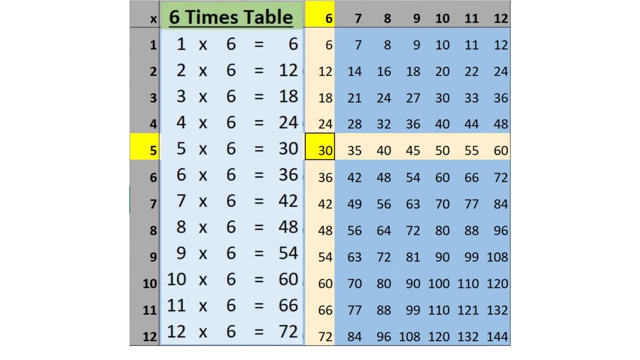 So the 6 times table answers are shown here. 1 times 6 is 6.. 2 times 6 is 12.. 3 times 6 is 18.. That's it, So that table is all in that column there. 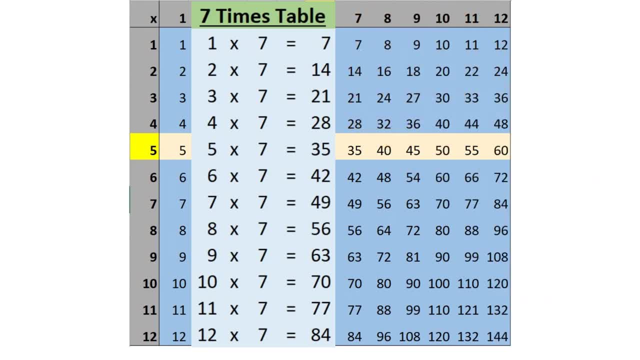 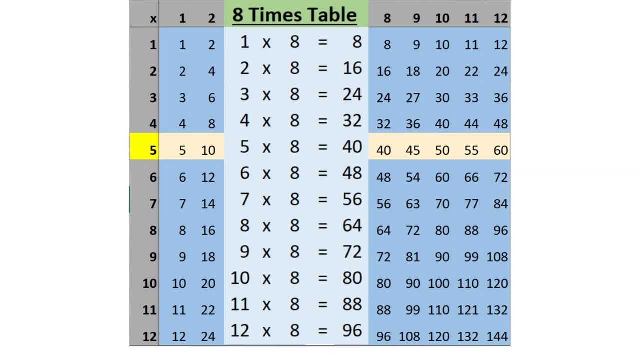 And the 7 times table answers are all in that column And the 8 times table answers are all in that column. That's why sometimes people would say: have you learned your times tables? Or they might say: have you learned the times table? 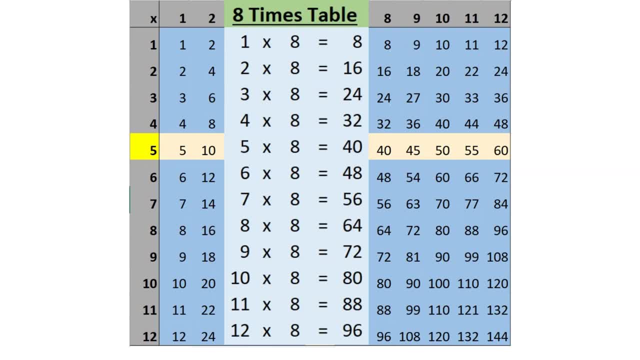 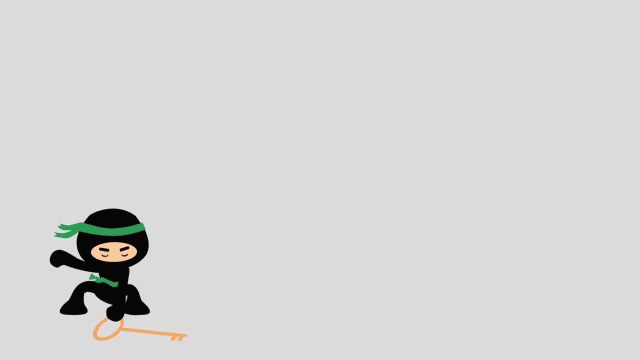 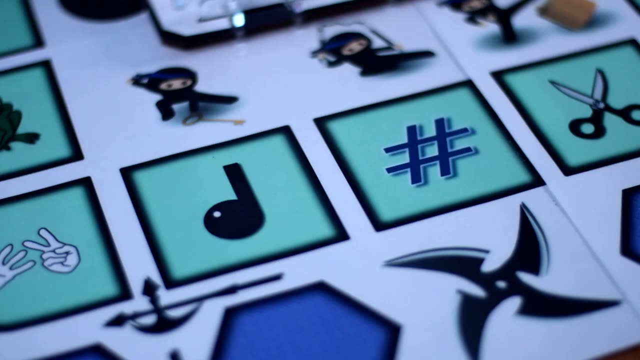 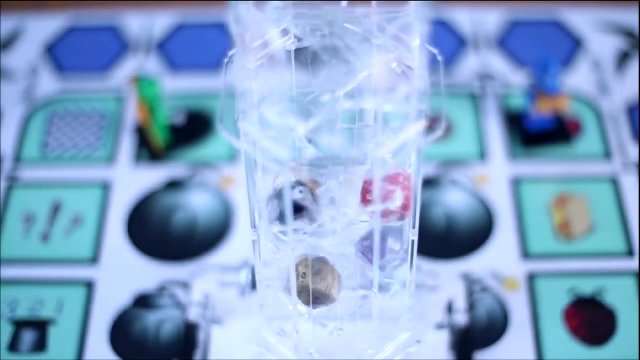 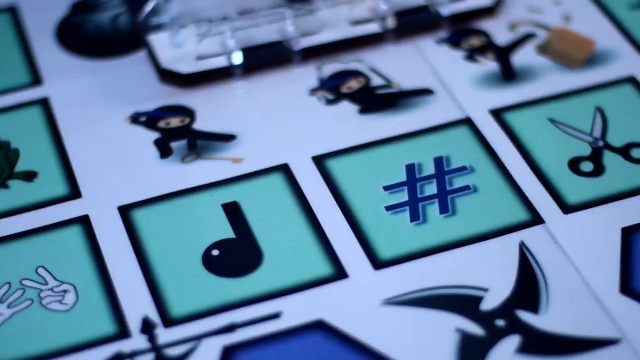 Or multiplication table, So you can call these times tables or multiplication tables. They both basically mean the same thing. That's what tables are. Thanks for watching. See you next time. Bye, Bye. 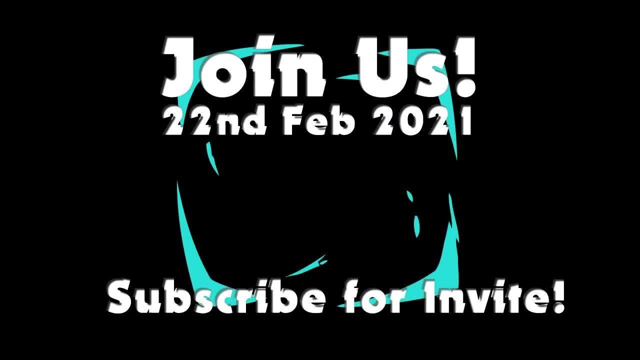 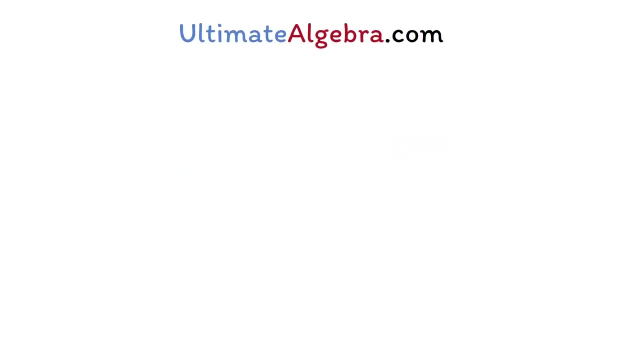 Welcome to another video from ultimatealgebracom. In this video, we will be looking at solving absolute value equations. We will use these 10 questions to teach you everything you need to know. It's very important that you watch the entire video for best results. 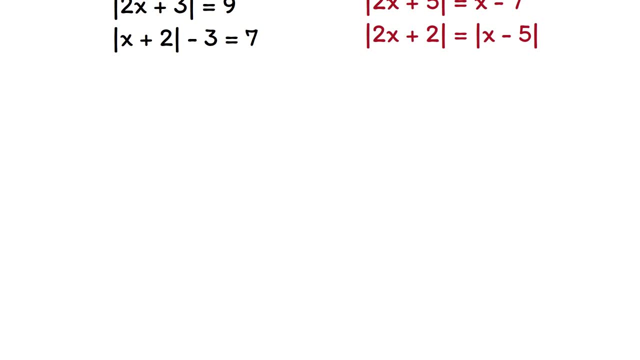 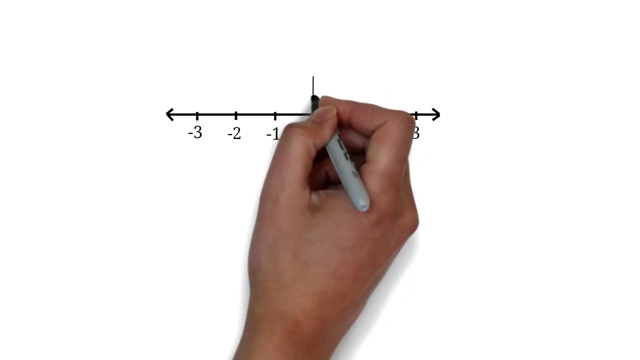 Before we solve the questions, let's look at what absolute values are. Let's draw a number line, So we have 1,, 2, 3, and so on. We have negative 1, negative 2, negative 3, and so on. The idea of absolute value is that it doesn't matter if you moved. 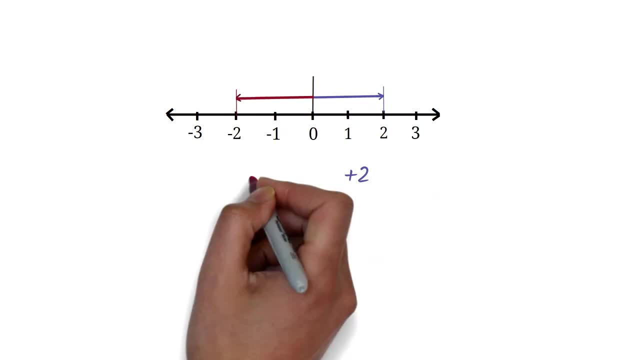 2 to the right to get positive 2, or you moved 2 to the left to get negative 2.. Absolute value is only concerned about the fact that you moved 2.. So we can say that the absolute value of negative 2 is 2 and also the absolute value of positive 2. 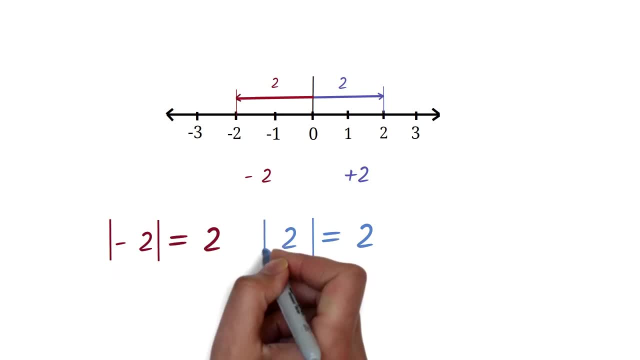 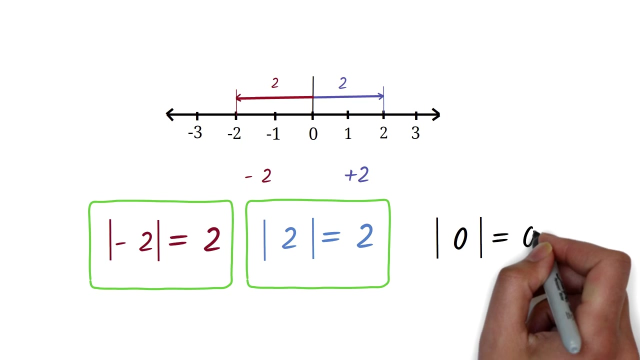 is 2.. Notice that we use these lines to represent absolute values. Absolute value is always positive. The absolute value of negative- 2 is positive, The absolute value of positive 2 is positive And also the absolute value of 0 is 0..